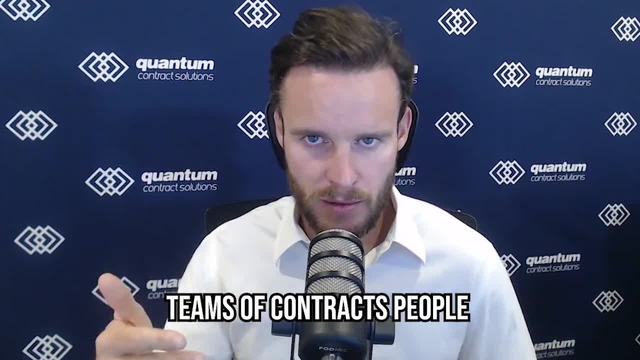 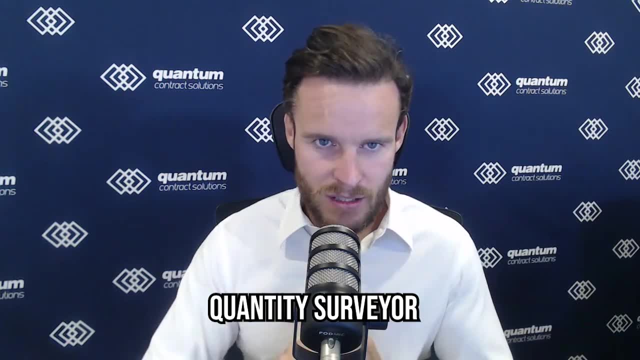 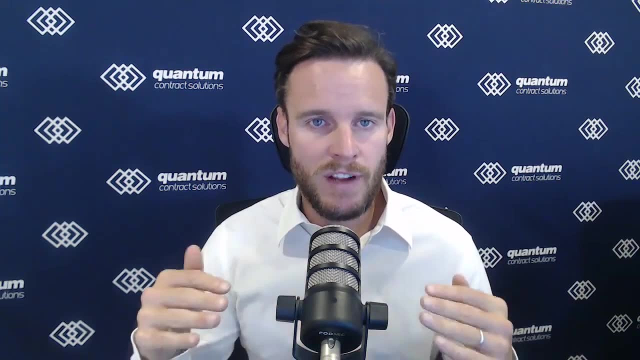 construction companies have teams of contracts people, so it can be different names for contracts people. they can have a contracts engineer, contracts advisor, contracts manager, a quantity surveyor. you can have a contract administrator. so lots of different names. really, most of them are doing roughly the same thing but with various different levels of skill sets. okay, and i'll explain that in. 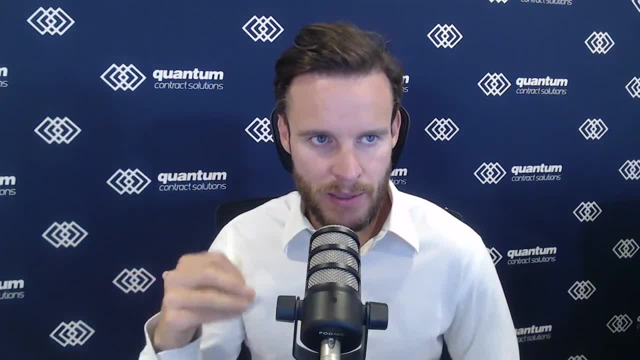 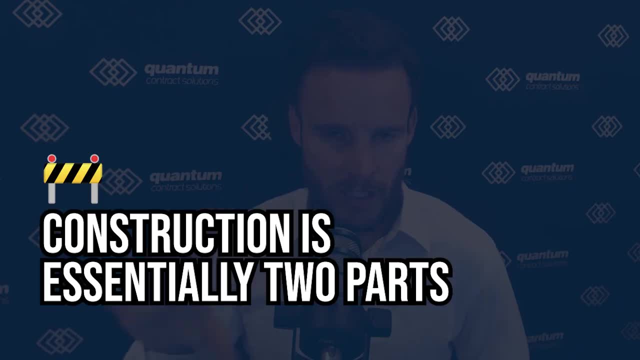 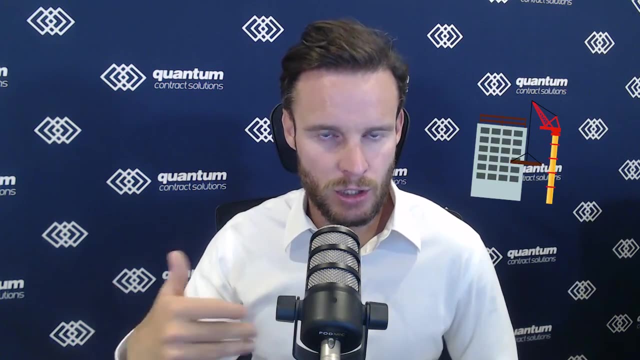 a second. so in the reason we need, the problems that we have in construction are basically this: that construction is essentially two parts. right, obviously it's a little bit more complicated, but in from a high level. one is you have to build the thing that you're, you promise to build, or 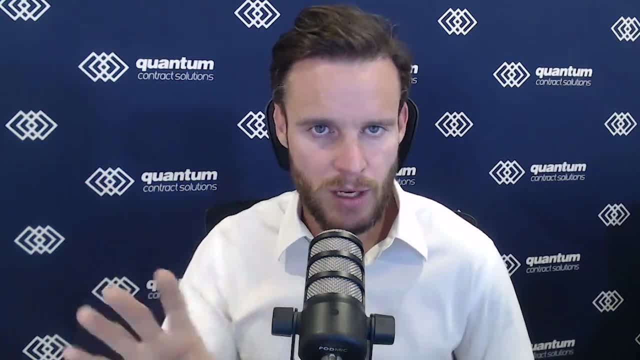 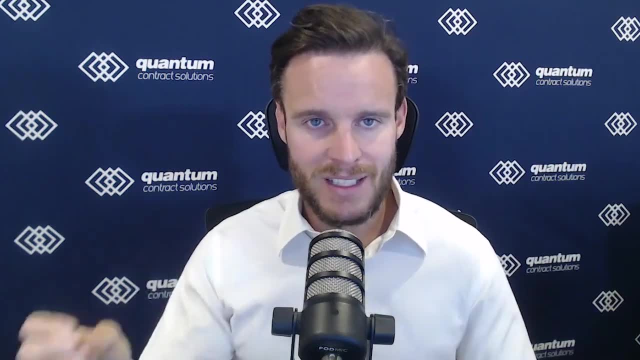 construct the thing that you promise to construct or deliver the thing whatever you've promised, right. so you've got to fulfill your obligation to deliver the thing that you've promised, to deliver the thing essentially, and that's obviously very, very important. but the second part of construction, 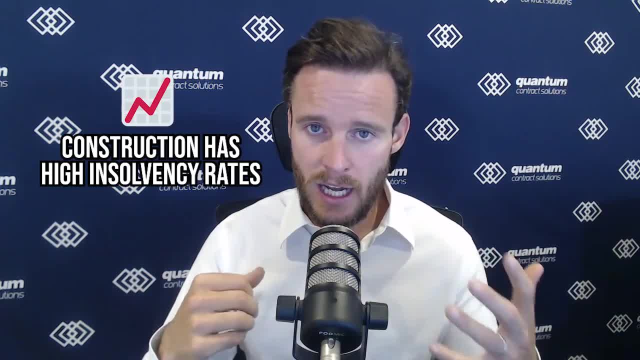 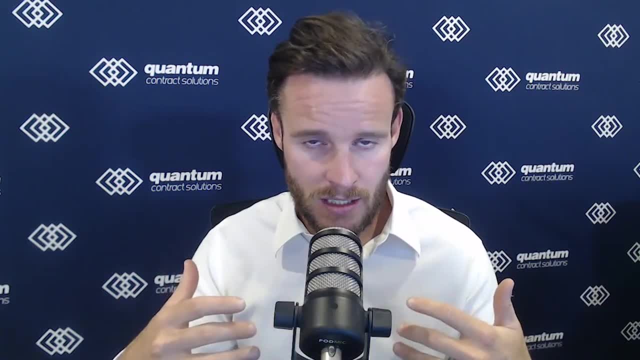 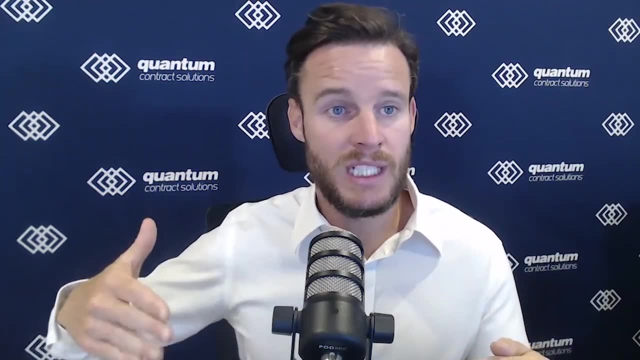 is getting paid now. construction has a really, really high insolvency rate, so it's 26 in most countries. it's roughly there thereabouts of all insolvencies comes from the construction industry, and this is because a lot of people don't understand that it is that important to get to be. 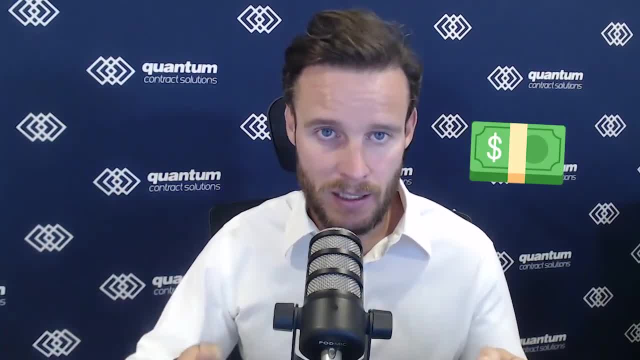 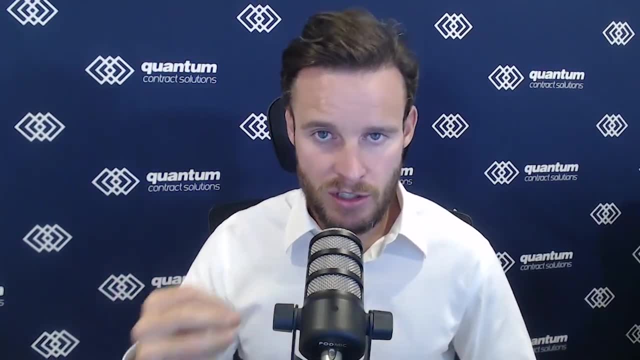 have your ducks in a row with regards to the contract to make sure that you get paid. now, everyone has different motivators, right? so, obviously, if you're a tier two constructor, so a subcontractor, right? i'm kind of talking to you guys. everyone in some capacity, except for the client, is going to be reporting up the way, so 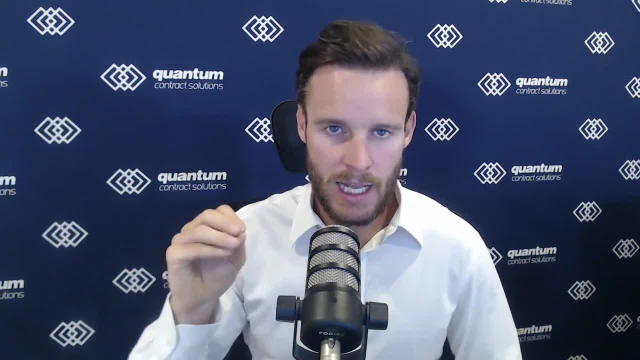 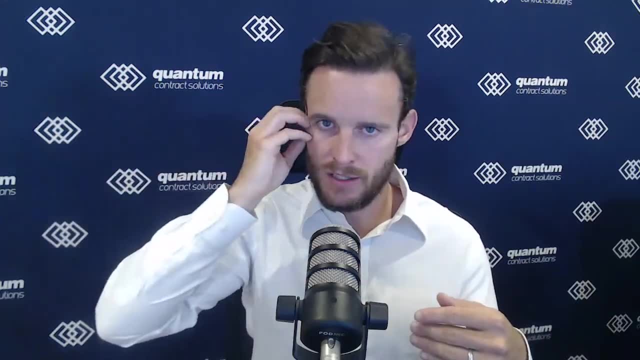 it applies to the tier ones as well: the general contractors, main contractors and two, but ultimately the people up the line have different motives to you. they obviously want to make a profit. they want to save their own costs and in the world we're living in now, if they can save costs by not paying, 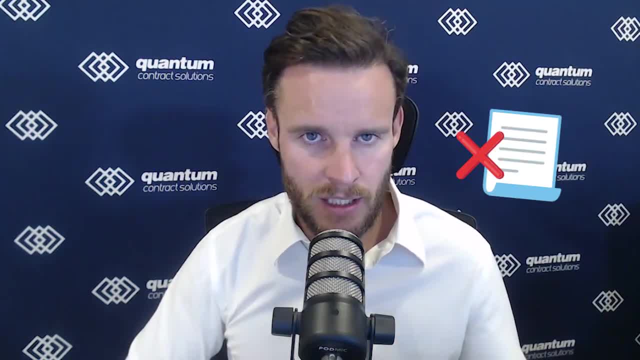 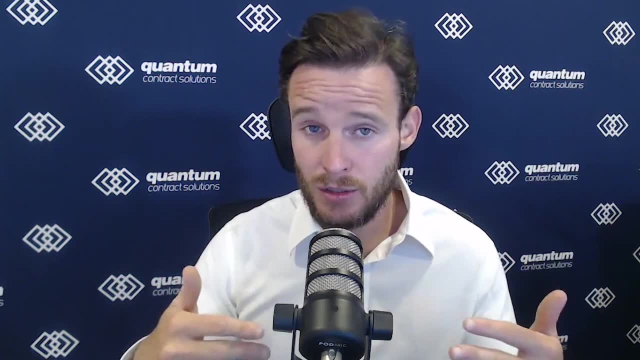 you for work that you've done properly because you haven't complied the contract. they won't if they can use you know if. if they can manage the contract in such a way that they can get you to fund most of the for them, they can have most of the cash you can do most of the cash flowing for them. 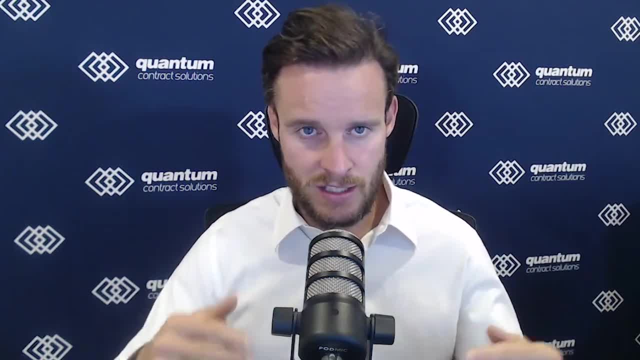 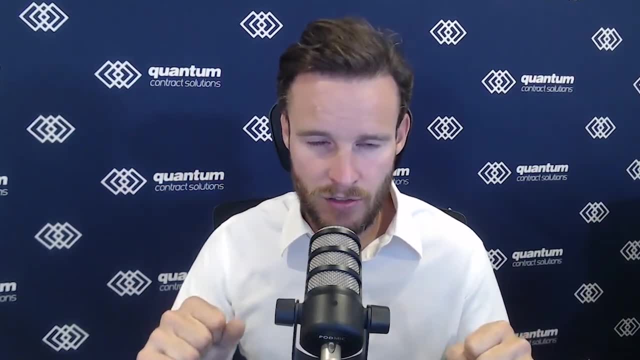 it makes their business better. so there's a lot of competing things that you need to understand. so you obviously don't want to fall into that trap where you're not getting paid for extensions of time that you've been delayed on like unfairly- no, no, fault of your own. you don't want to be in a 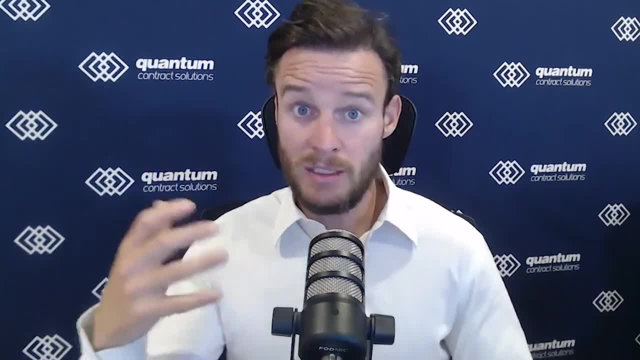 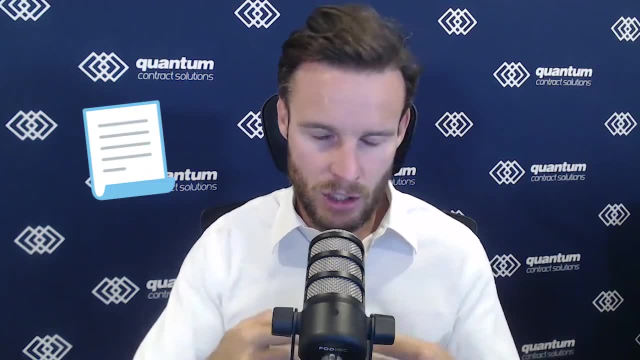 situation where you're not getting paid for your change orders, you're not getting paid for proper work, but you're not getting paid for your future. but you're not getting paid for your future. there's not a lot of people in the world wanting to push their will onto you, right? so you need to be able. 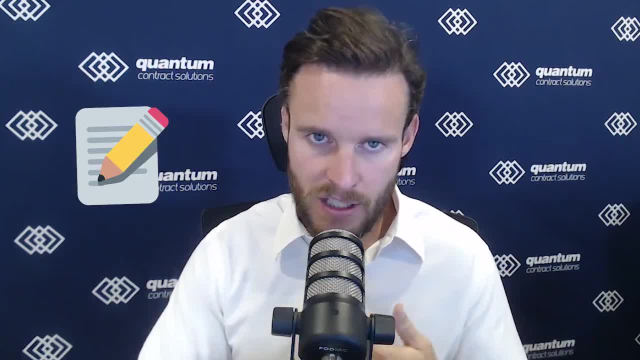 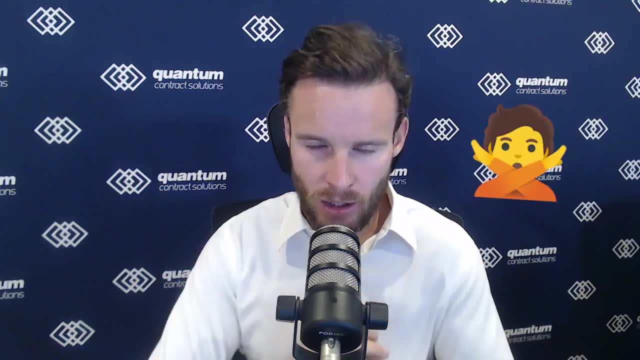 to understand the contract and push back and understand that the best and biggest construction companies have contracts teams for a reason: it is to sign a lower risk contract, it is to have better cash flow, it is to make sure that you get paid and it is to ensure that you avoid disputes at all. 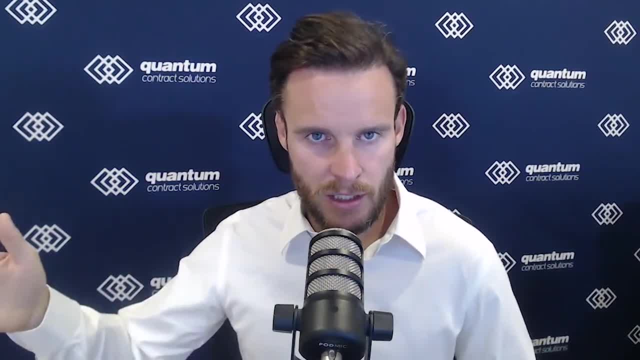 costs. okay, now this is where the contracts administrator comes in. contracts administrator- what he's going to do a really good. so i've given you a list of the different company, uh, the different types of people, but i'm going to give you the their job for you. 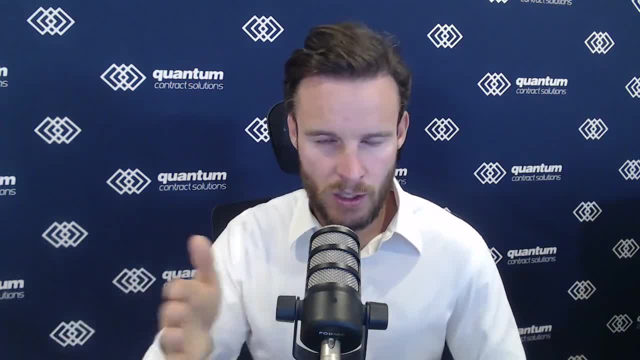 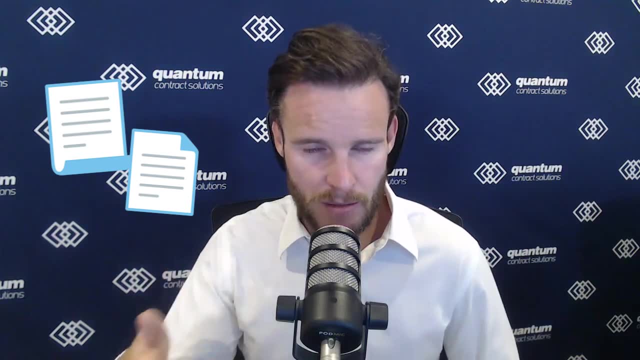 start to finish right and and depending on what, like where you are in in the chain, but generally a contracts administrator might help with your contractual documents and your tender or bid submission. okay, he won't do the estimating. i i wouldn't. i wouldn't imagine he will help put the. 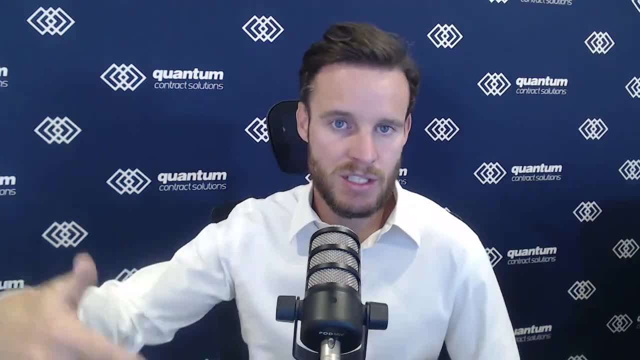 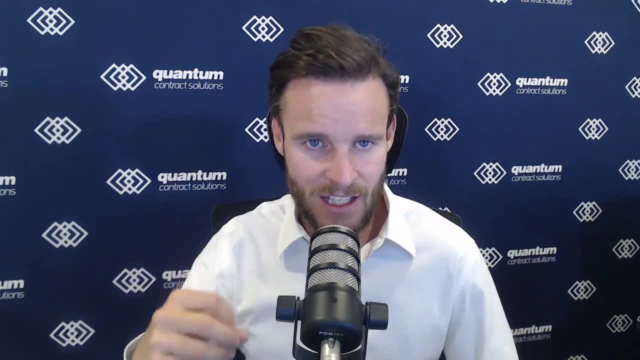 documents together. he or she will help put the documents together and submit them to as part of your bid or look for work. essentially, then, you're going to get given: yeah, you're going to be part of a tender. as part of that tender that you're the bid that you're submitting, there's 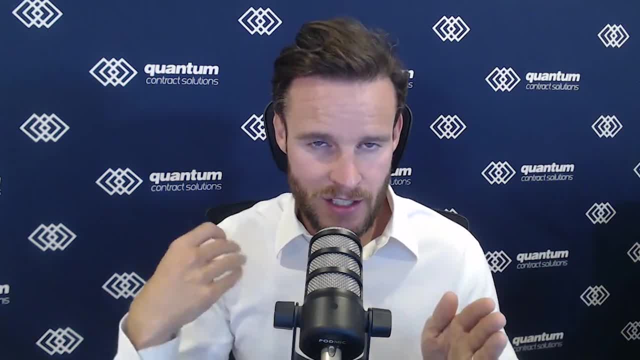 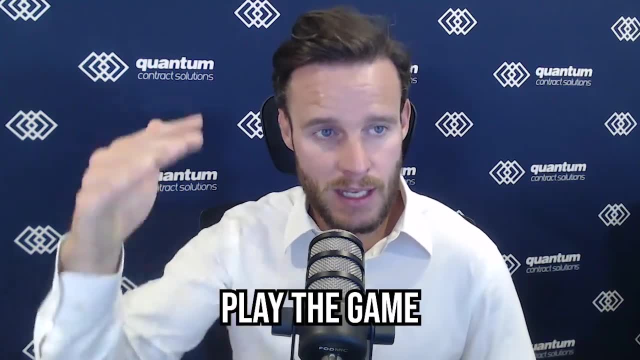 going to be a contract in there. in that contract, they have essentially given you their worst terms and conditions possible, and so what you need to do is play the game and you need to say: hey, here are all the things that we don't agree to. now, honestly, from having done over 2500 of these, 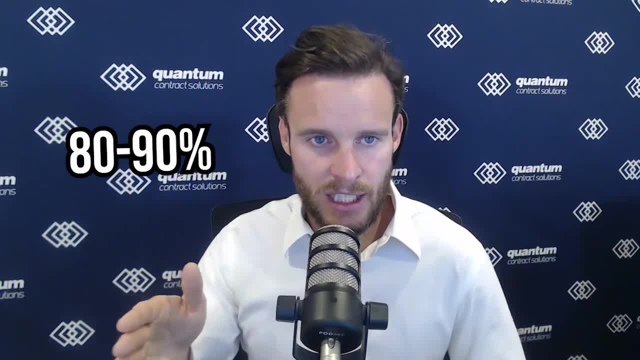 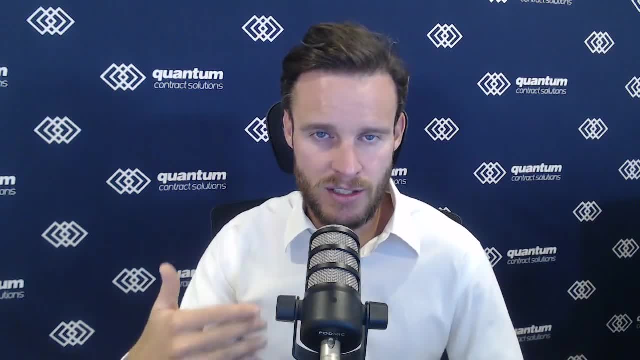 in the, in the, in in our business. you can get 80 to 90 percent of these to what you asked for across the line. they are expecting you to negotiate. if you think by not doing it you're doing yourself a favor, but you're going to look easier to deal with, you're not? they look at you. 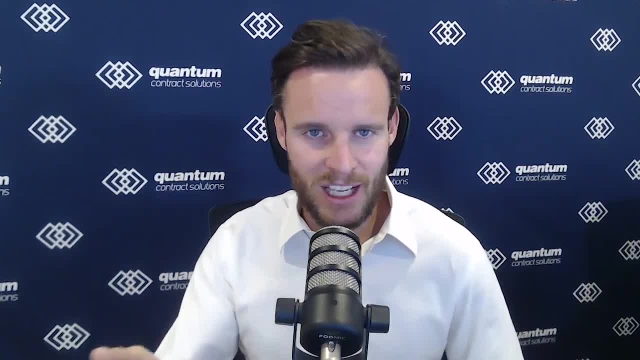 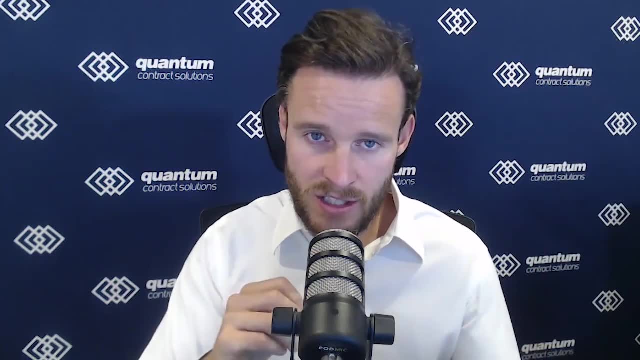 and they think you're, you're green, you don't know what you're doing. why is this guy not like pushing back? right, because everyone pushes back, so push back. you'll get 80 to 90 percent of things across the line when you go. when you understand what to negotiate in the contract you're going to. 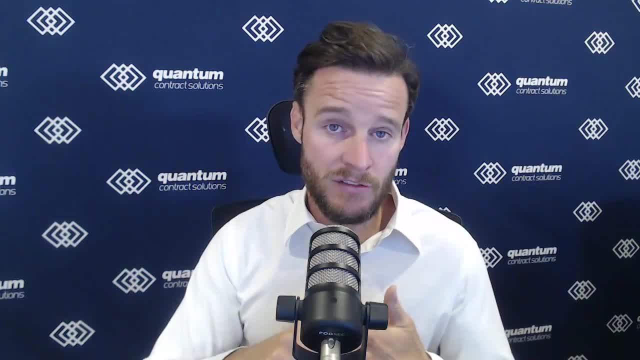 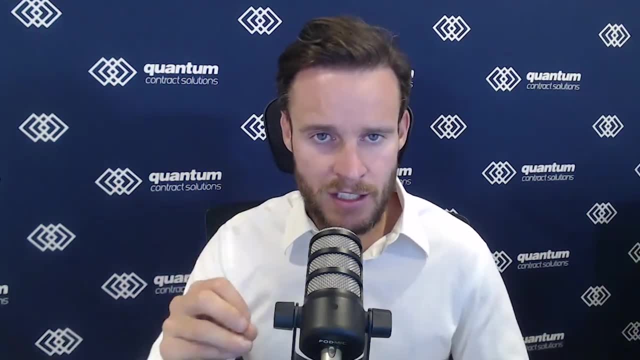 the risk is going to be way, way less. you're going to set yourself up to have better cash flow during, during the, the construction and generally you're going to set yourself up to be more and more successful. so that's on the front end. so that you need this: the contracts. 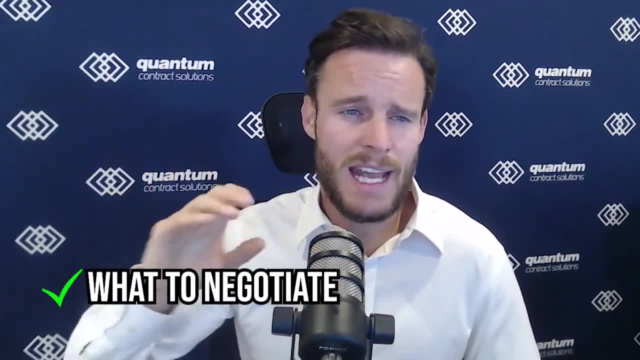 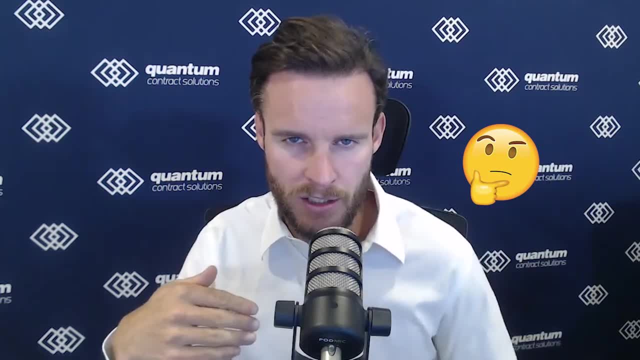 administrator needs the skills to understand what's in the contract, what to negotiate, how what i negotiate impacts the project right. what to bother negotiating for. what to what not to bother negotiating for. you've got a contract administrator that can do that. it's very, very powerful, a very 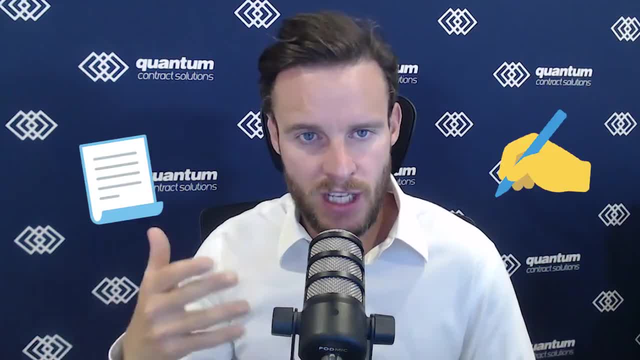 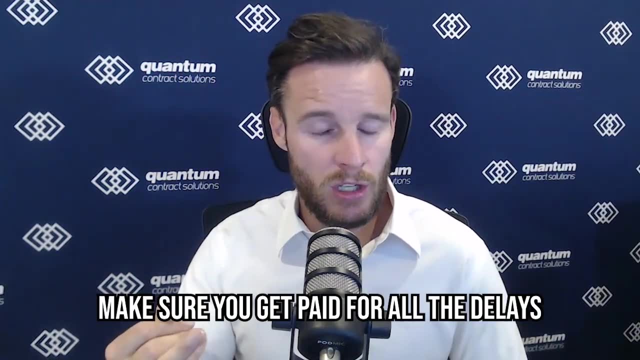 very good contracts. a person in post award, all right. so you've signed the contract. now you've got to. essentially, there's there's three things you got to do, right. you've got to make sure that you get paid for all, all of the delays that are not your fault. so you're going to document them. make sure that you're following the contract, to make sure that you're you're compliant, so that you get paid for the delays. you don't want to take on someone else's delays. you want to make sure that you get paid for all the additional work that you do. this is where 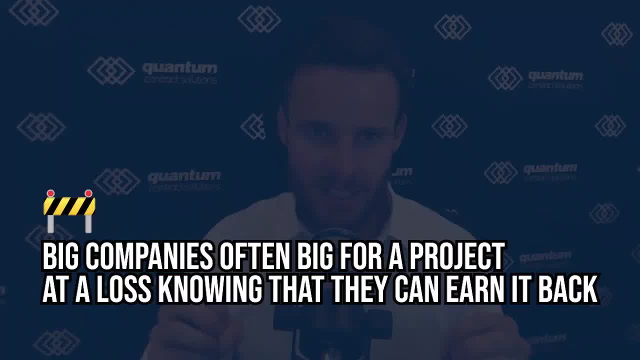 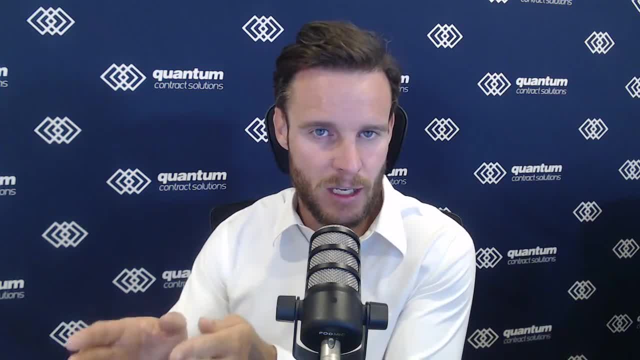 the money is right. so you please understand that the biggest companies- oftentimes they will bid for a project at a loss, knowing that they got this part of the business sorted and they're going to make up all of their profit in the post award phase. so you got to get that. that's where the 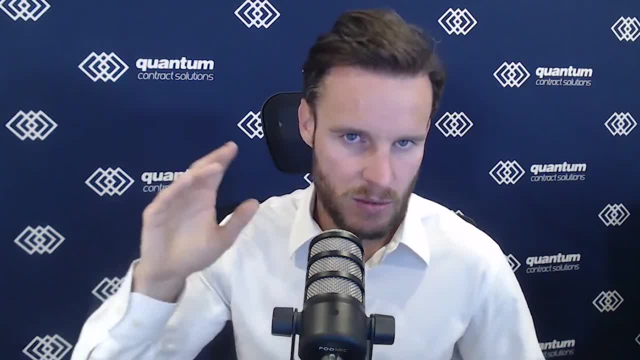 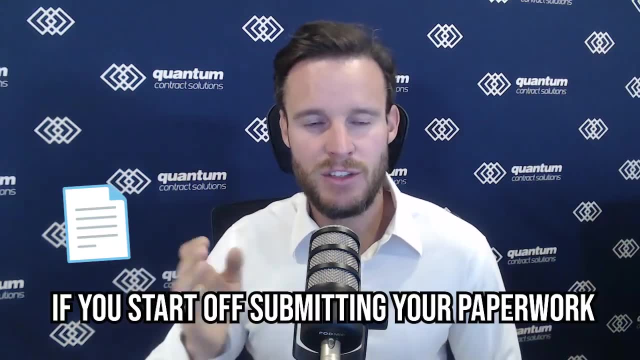 money is. so get your variations, get your changers- eots, whatever they're called in your contract sorted. get them get that process like clear as day, perfect, okay again. if you start off submitting, they're just going to think you're very professional, you know what you're doing. if halfway 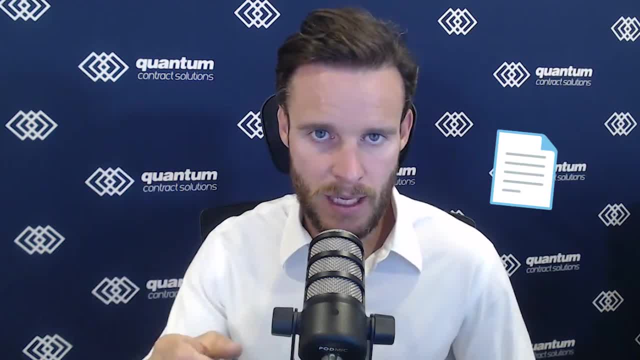 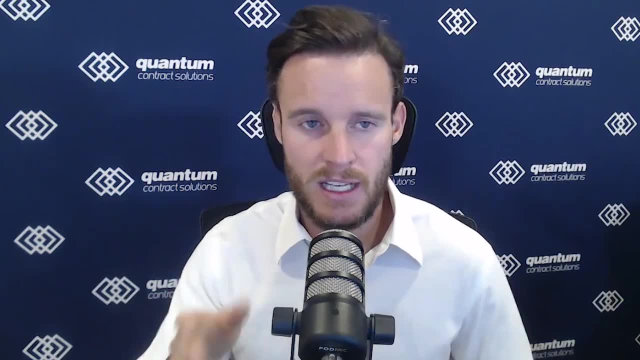 through the project. all of a sudden you're like, oh, we're not getting paid for stuff, we're going to start submitting paperwork. they're like, whoa, what are you submitting all this paperwork for? so start professional. and they'll think, oh, these guys are very commercially savvy, they're very good, okay. so 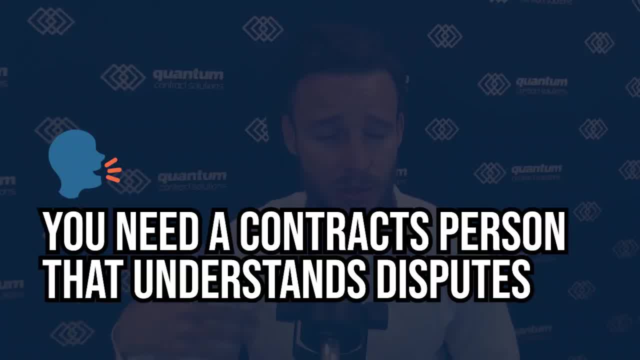 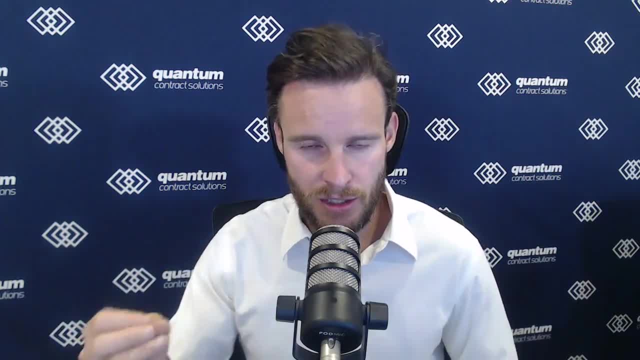 that's the first thing. now, at the end, you need a contract person who can understand disputes, and so, when you understand what to do next, what's the strategy of a dispute that makes a huge difference to your company? now, there's lots of dispute experts out there. there's a lot of lawyers out there. the i. 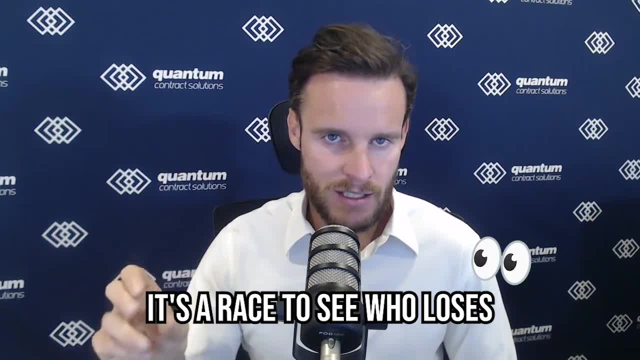 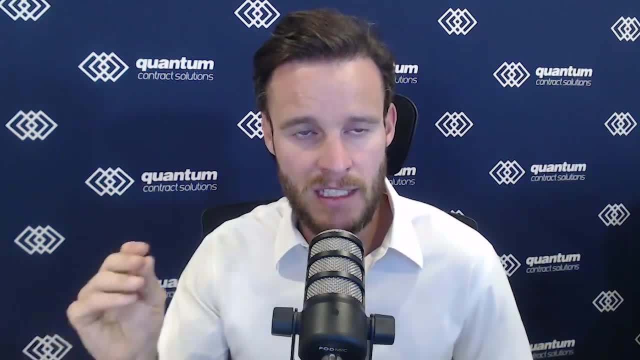 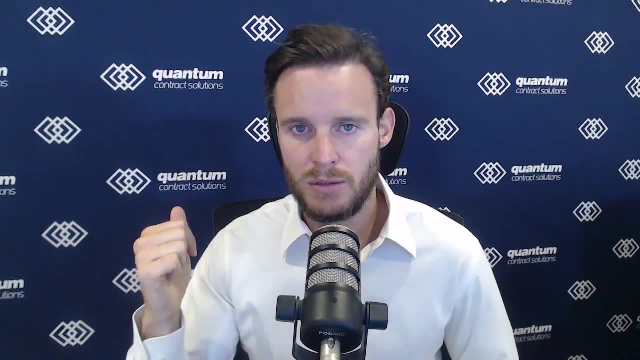 to you that if you're in a dispute, it is a race to see who loses the least amount of money. nobody wins in a dispute, so avoid disputes at all costs, even take a hit. it's worth taking a hit to avoid a dispute, small hit to keep the relationship to. yeah, get a resolution, get money into your. 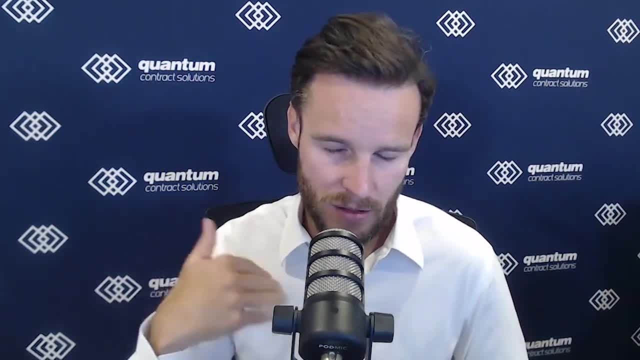 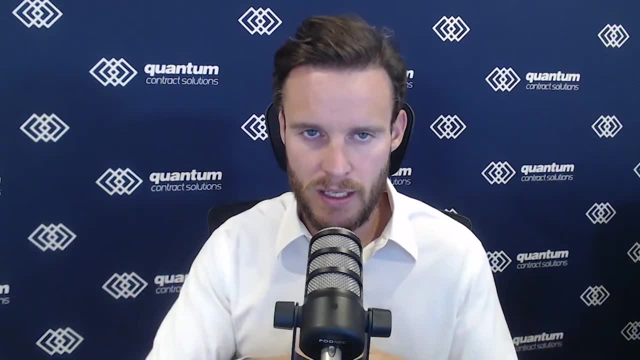 bank account quicker. it's definitely worth doing that. so you want to be able to devise strategies, to be able to negotiate a settlement of some kind, to get it done, you know, in a normal way, organized way. so if you can get a contract administrator that has those skill, set, that 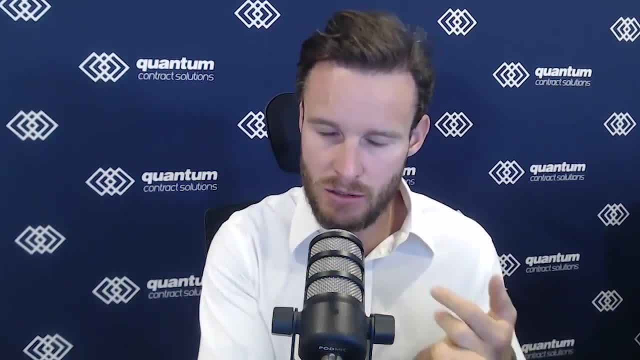 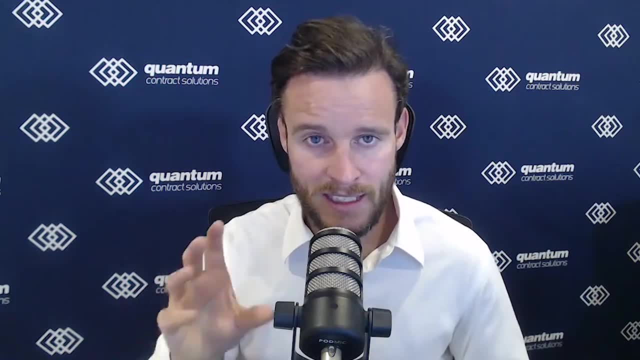 one can negotiate contracts in the front end. they can do all the paperwork during the contract and can make sure that they can give you the contractual advice and help to make sure that you avoid the dispute. you're on to a win and that's if you're look, if you're a contracts administrator.